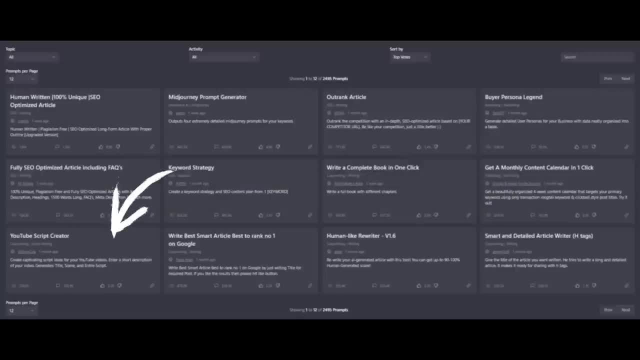 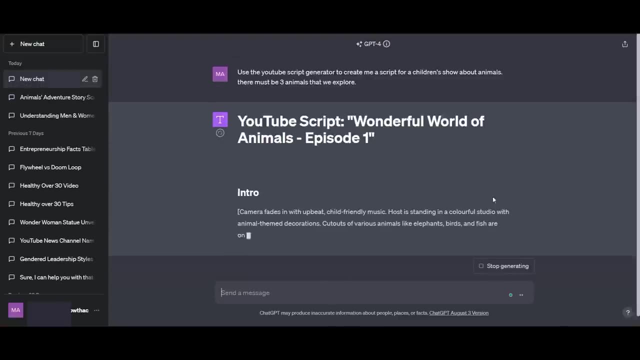 And what you're going to notice now is that you can use the script function. So we're going to ask ChatGPT to create a children's script for us. for a show about animals. There must be at least three animals to explore And ChatGPT 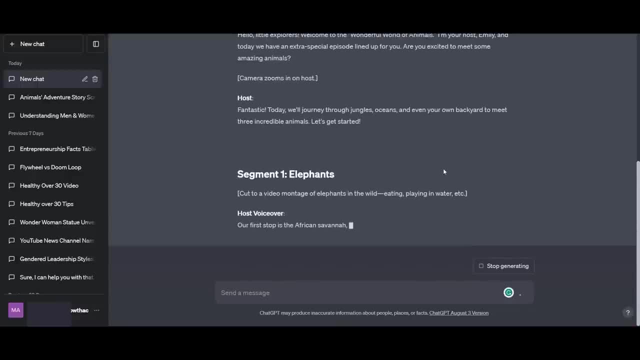 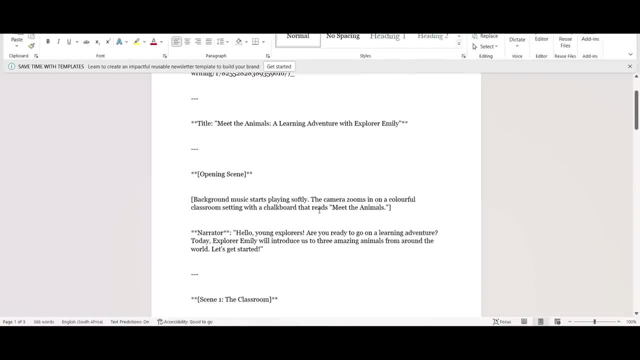 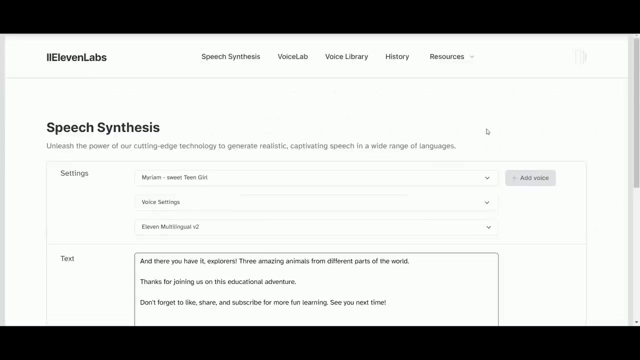 is going to do a great job of giving me the script. What I'm going to do next is I'm just going to copy this over onto a Word document, because that's going to be a lot easier for me to use. Then I'm going over to 11labsio for our voiceovers. 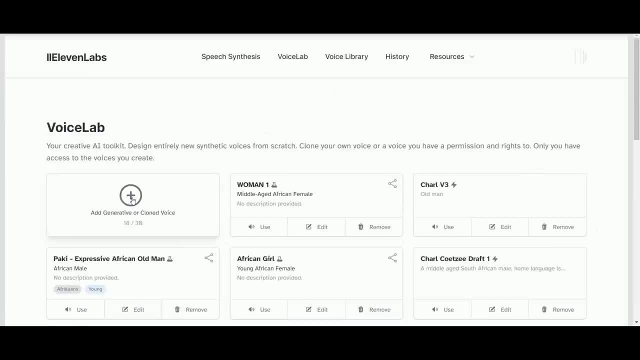 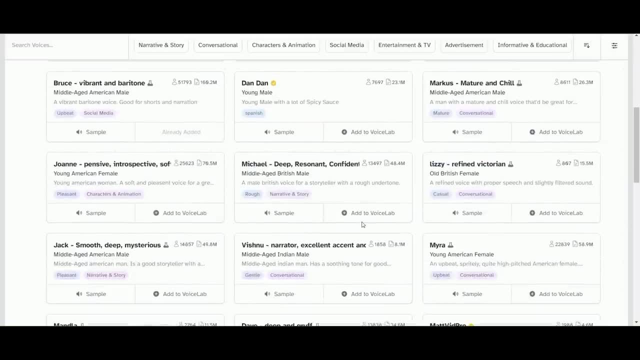 The cool thing about it is if we go to VoiceLab we can go and find the kind of voice that we would need for this children's show. So if we go to Voice Library, it's going to provide us a whole lot of choices here. We want something that fits the childish kind of theme, So let's look at some. 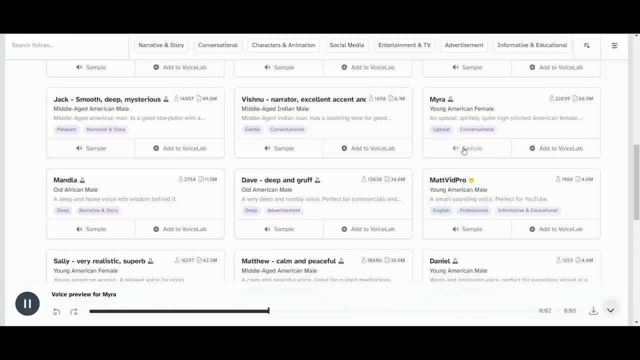 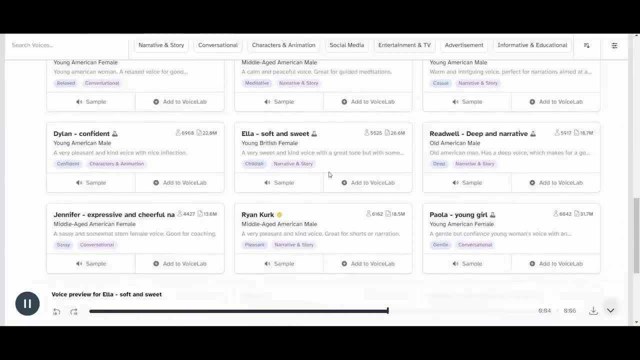 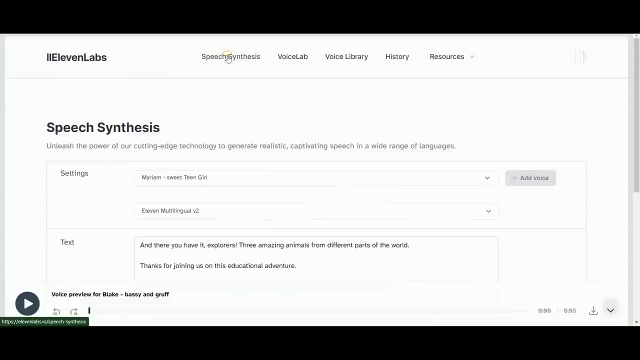 of the options here. The only thing to do with good advice is to pass it on. It is never of any use to oneself. Kindness is more important than wisdom, And the recognition of this is the beginning of wisdom. Once you find one that you like, you can then save it If you head back to your main page. 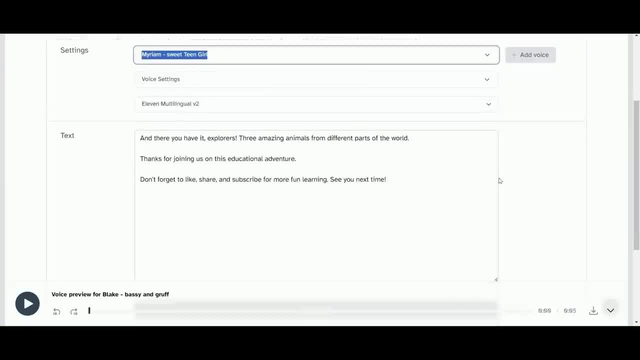 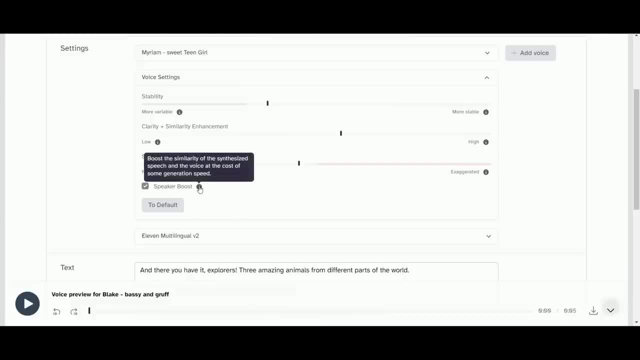 your speech synthesis page, you'll be able to, in the drop-down menu, choose the one. Next, we are going to change the settings. Just make sure we're happy with them- The kind of voice that we're looking for- And then after that we're going to input the first. 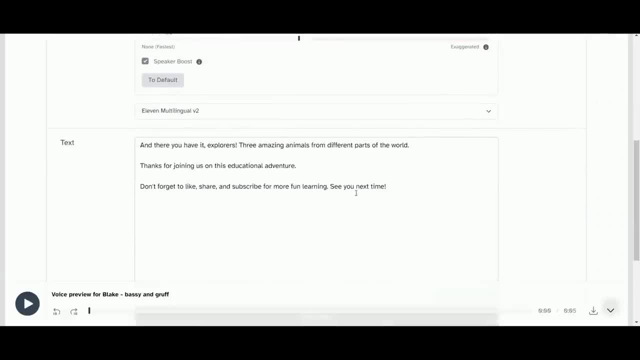 piece. Now we're going to go piece by piece, chapter by chapter, because we need about five scenes for our story. So what I'm going to do is I'm going to go to the first piece, And I'm going now is I'm going to put in the first piece, And let's listen to how that sounds. 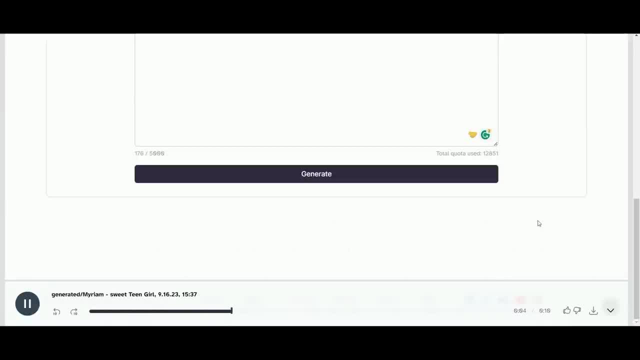 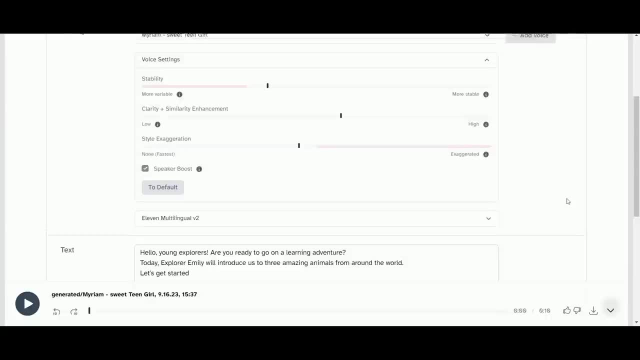 Hello young explorers. Are you ready to go on a learning adventure? Today, Explorer Emily will introduce us to three amazing animals from around the world. Let's get started. Okay, there's a few changes we need to make. Once we're happy with that, we can go ahead and. 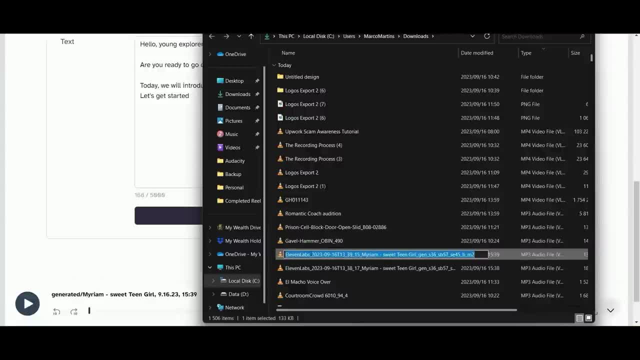 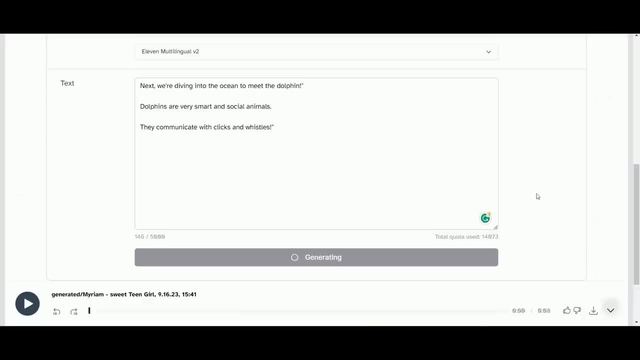 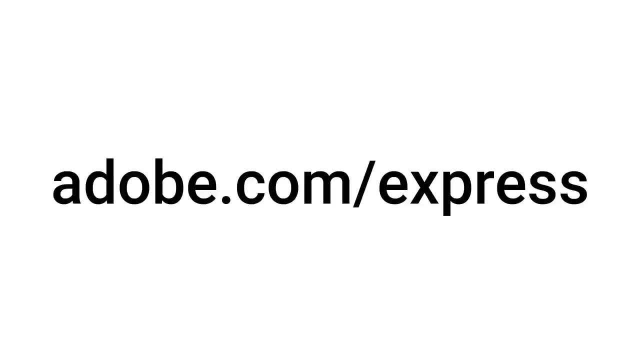 download it And I'm just going to rename each piece And then I'm going to do the same thing for each other scene that I have created here. After that we're going to go to adobecom forward slash Express, And this is the Adobe Express page. 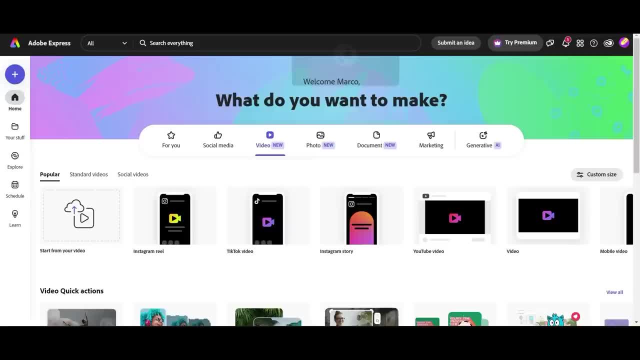 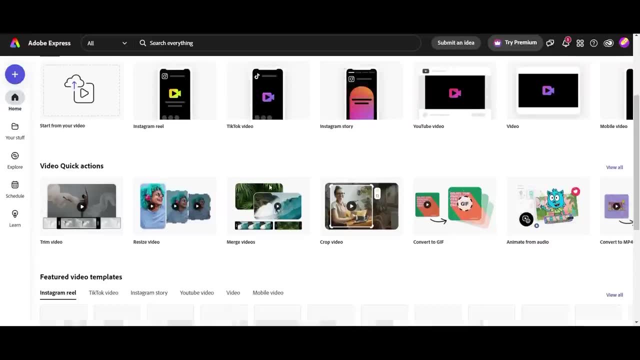 Now the cool thing about it is everything we need to create. our character is going to be right here, So what we're going to do is we're going to scroll down a little bit In the video functions, we're going to look for quick actions, And you'll see this. this animate from audio function over: 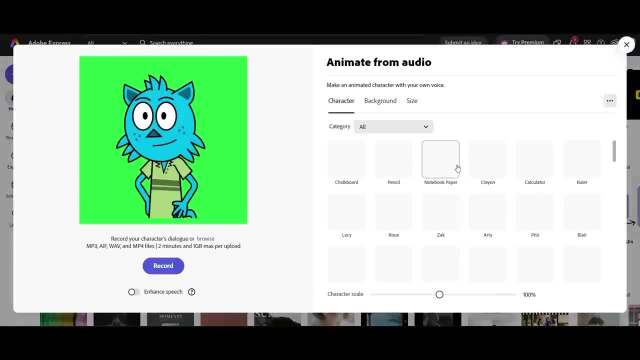 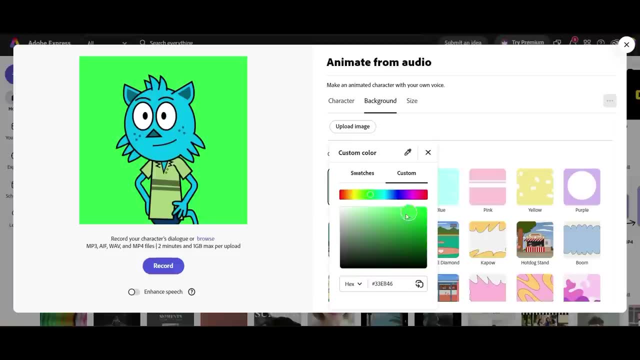 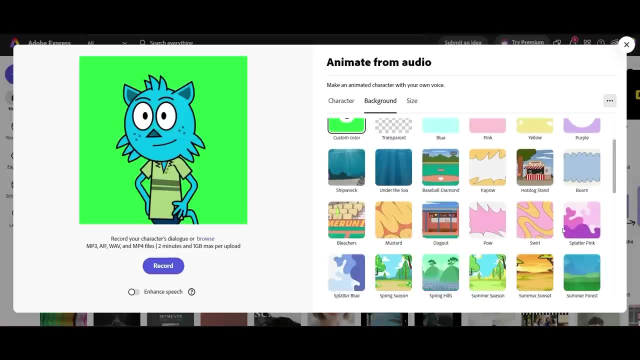 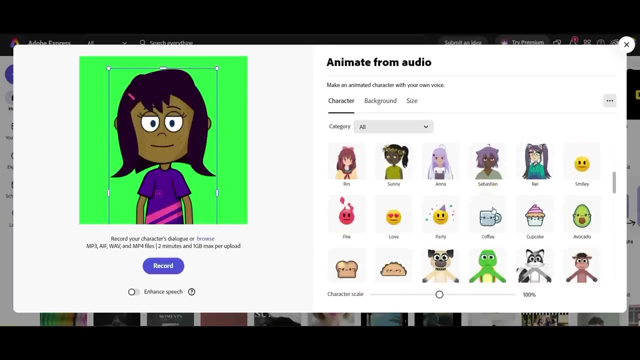 here, So we're going to click on that. First thing we need to do is change the background color. we need a green screen background, And then we have a whole lot of different characters that we can play around with here- Some really, really interesting characters for our animation. Once you find one that you'd like, we're 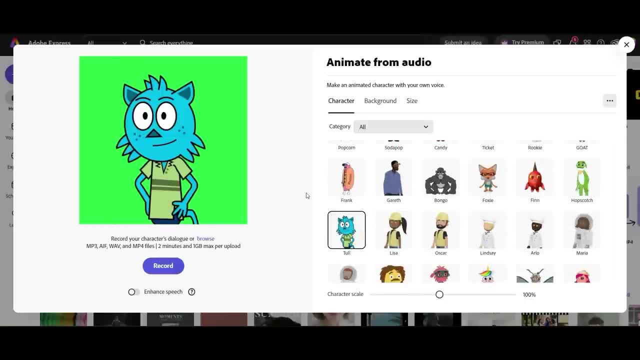 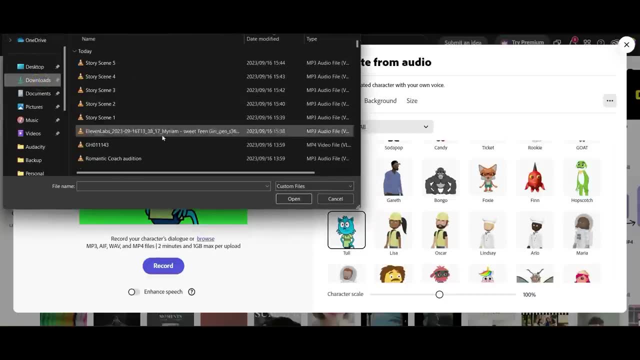 going to go ahead and choose, tell And you're gonna see over here. it has the Browse function we're going to put in our first scene over here And in a moment it's going to produce it. So let's see how that. 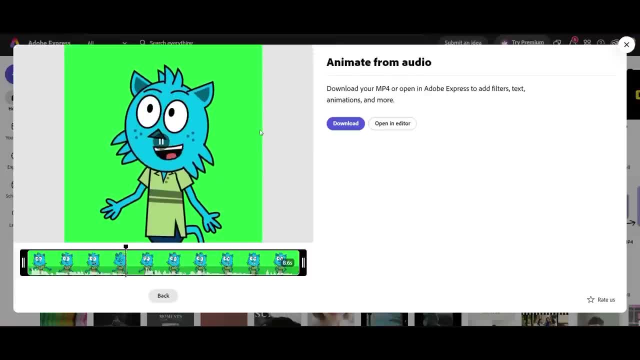 sounds. Hello, young explorers, are you ready to go on a learning adventure? Today, we will introduce you to three amazing animals from around the world. Let's get started. Well, that's actually pretty cool, So we're going to go ahead and do the same thing for each one of our 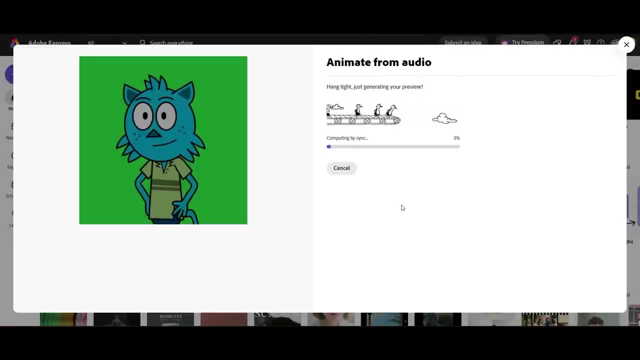 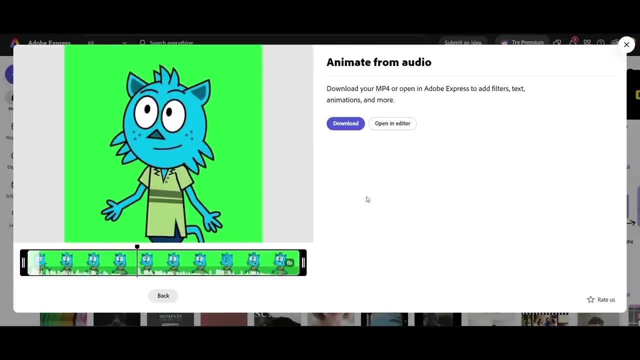 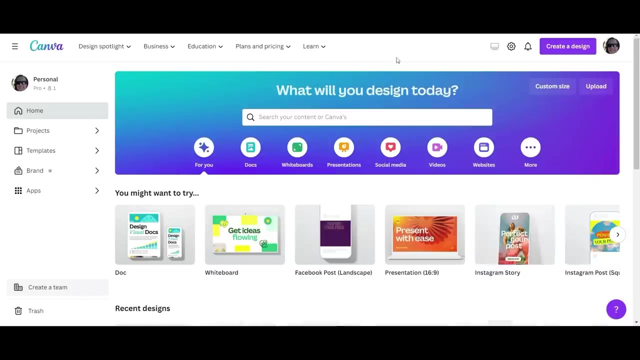 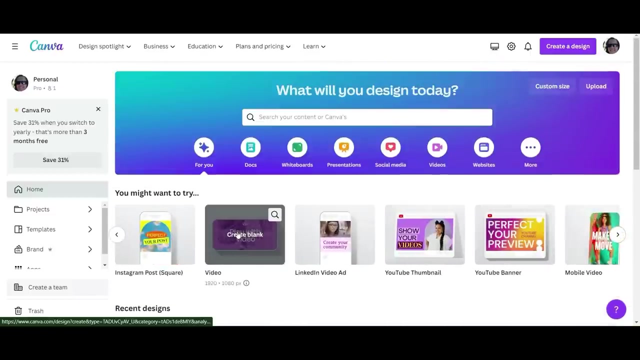 scenes And then after that, we're going to go to canvacom. So now that we've we're in Canva, you're going to go to the video functions, you're going to look for the video landscape function And we're going to 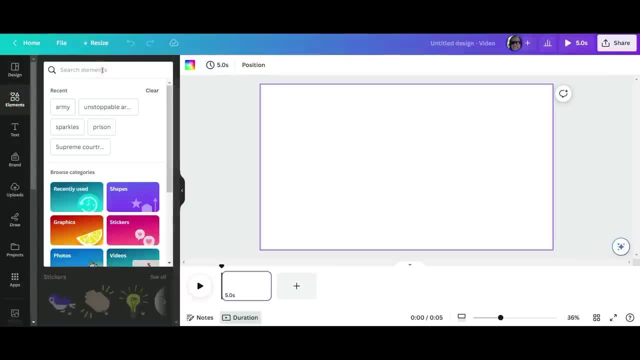 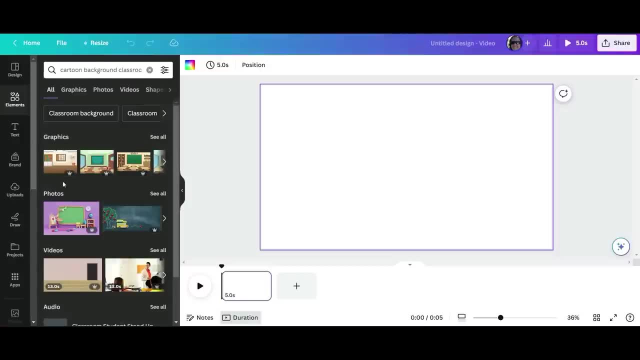 go to elements here And now we're going to look for a background. So I'm going to look for a cartoon background classroom. If you have Canva Pro, you'll have access to the pro images. If not, that's okay, you'll find something. 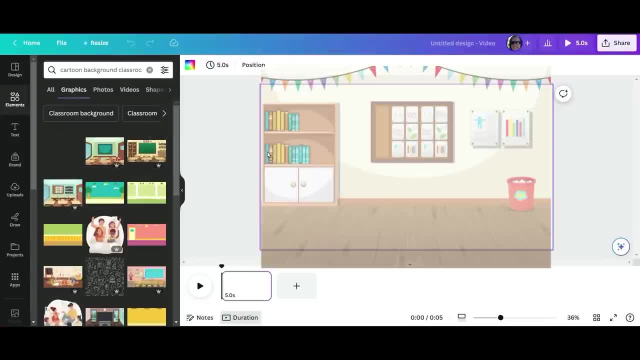 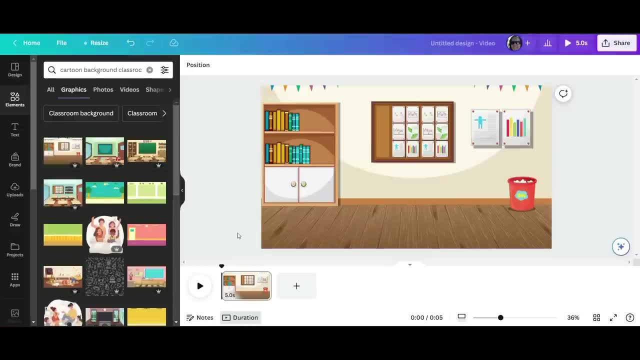 that you can work with. So, now that we've created this, this is a simple, clean background for what we need to start our video off with our character. First thing we need to do is have a look at the timeframes for each one of our 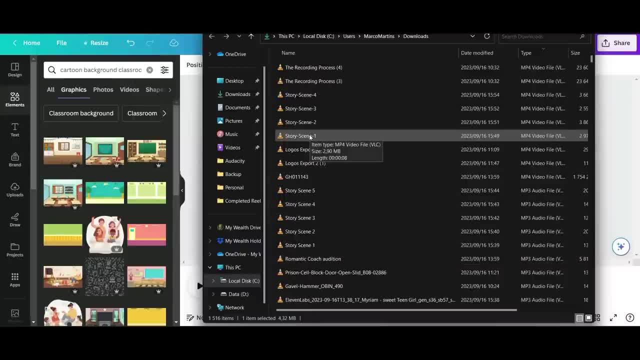 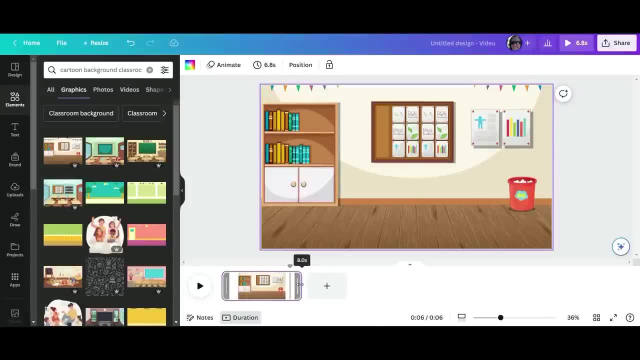 videos. So if you look at your videos, it'll give you the time. So we're going to go ahead and change up the setting to be exactly the same timeframe, So the first one is going to be eight seconds- Great stuff. Then I want to show you what Canva can do in terms of just creating. 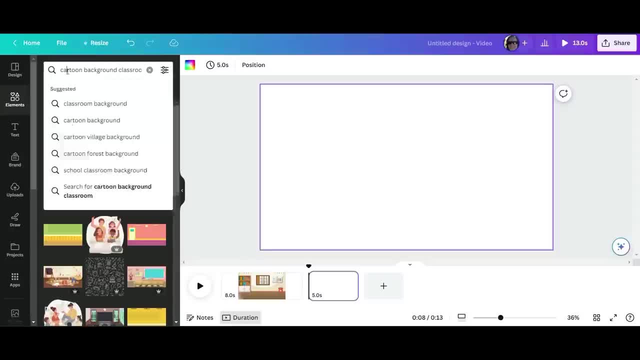 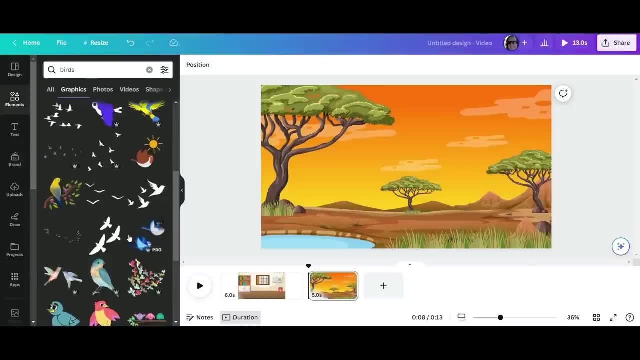 really cool, fun animated backgrounds. Our next scene is going to be about Africa, where our elephant is going to be, So we're going to look for some birds to put into our image. Now, I've tried this first one, not great, But let's go in to see if there's others. Oh wow. 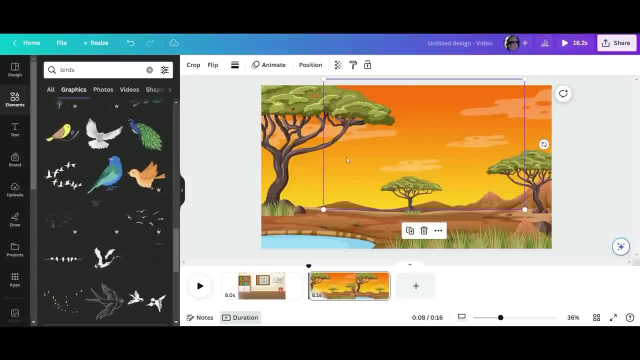 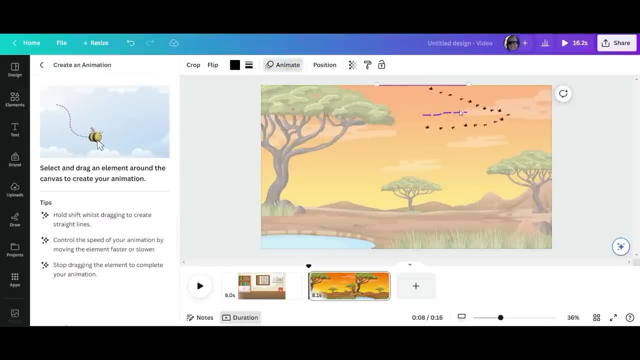 bird formation flying in front of me and flying V. Now it's already animated and it's moving. But if we go to animate we can actually create a kind of track for this animation to follow. And if you just move it, click on it, move it. that's what's going. 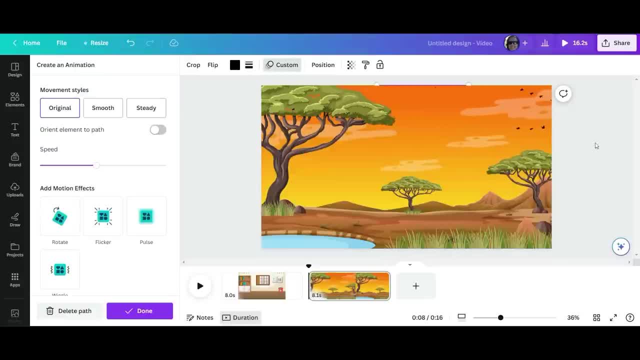 to happen in your picture. you can decide if you want it to be original, smooth or steady. Smooth just means it's going to smooth the motion. we can also slow down the speed, So this is where Canva is incredible. So let's go ahead and add a few more details in. 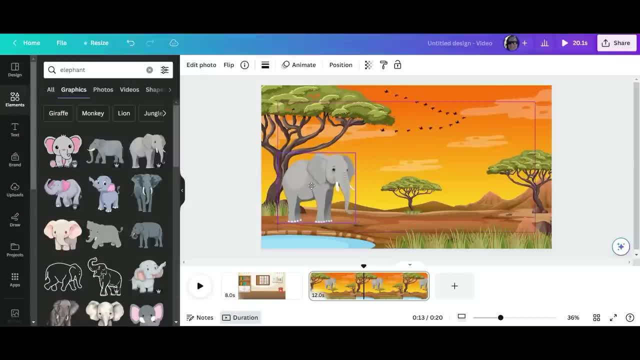 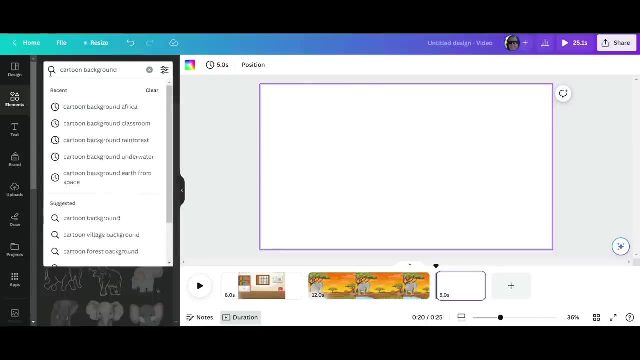 Let's look for our elephant. So we're going to put our elephant into the picture, maybe play around with the animations, or even if we just wanted to keep still, that's fine. And now we're going to do the same thing for the rest of our scenes. 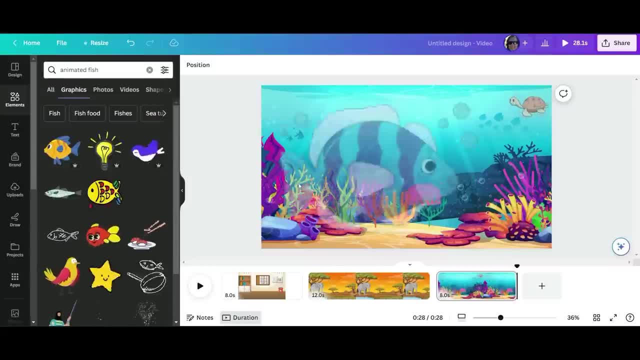 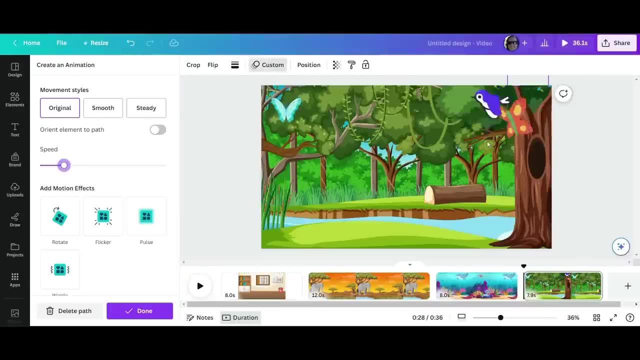 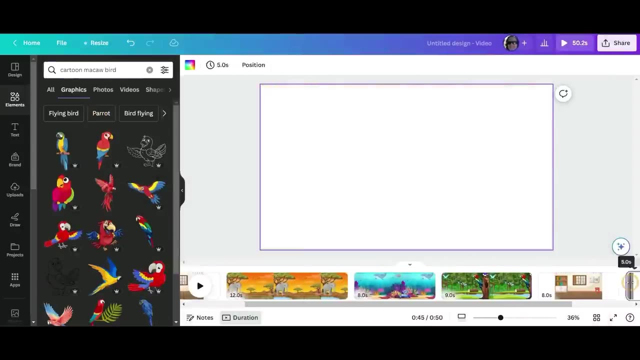 Canva is blowing me away with its functionality right now. Canva will still operate, so it won't stop shooting. once we've created our scenes and we've made sure that we've adjusted the length to be exactly the same length as our audio, the next thing we're going to do is go over to filmorawondersharenet. 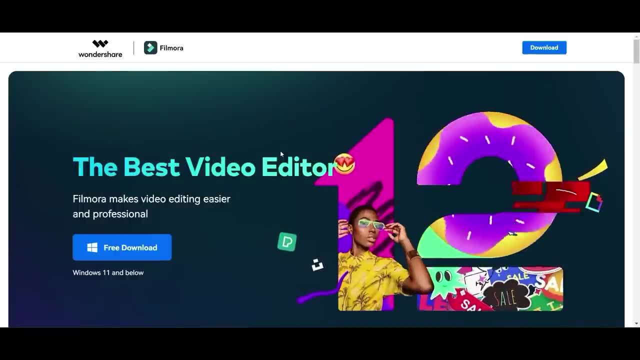 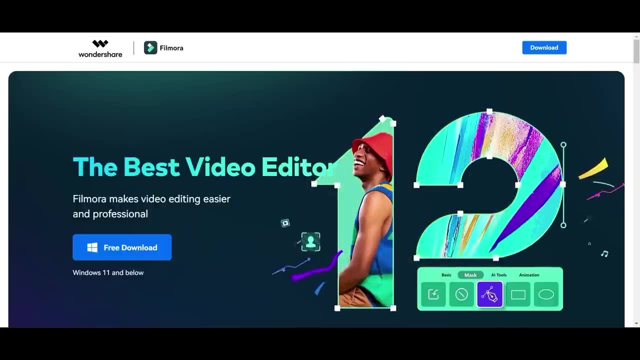 and, don't worry, all the links will be in the description below, and what you're going to do is you're going to go and download it for either your mac or for your windows pc. once you've done that and you've set up your account, this is going to be your dashboard, so we're going to import all 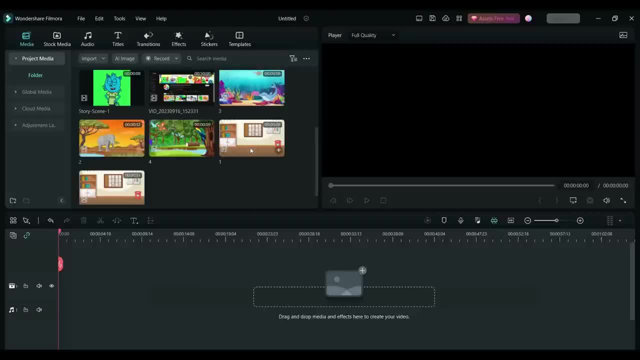 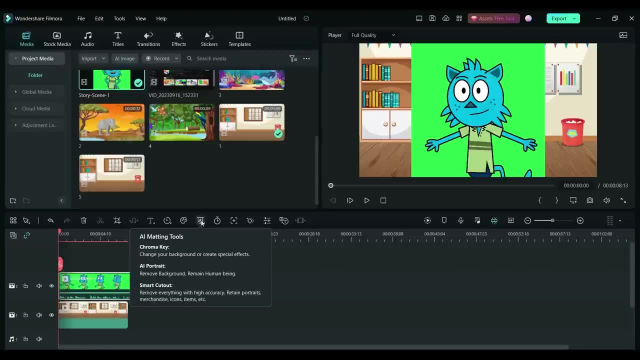 the information, great stuff. so once we've done that, we are going to take our first clip, we're going to apply it there, and then we're going to take our character and we're going to put it right over the top. okay, so first thing i'm going to do is i'm going to access the chroma key function. 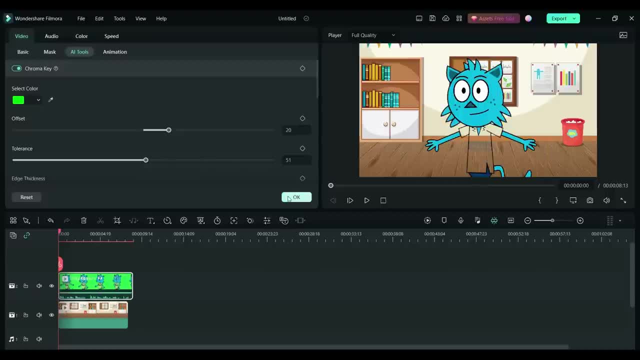 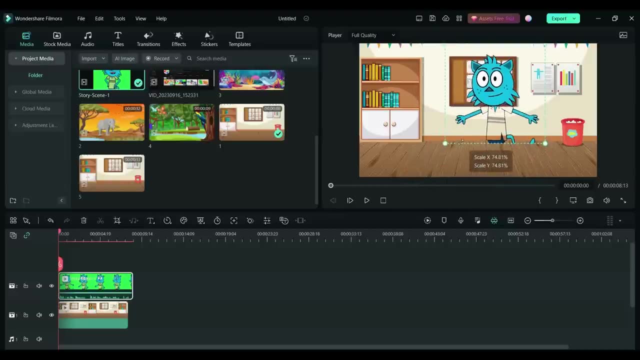 your green screen will disappear. now what we need to do is: there's the shirt is a little bit off color because it was there was a little bit of green in it, so we need to go and play around with that. so let's head over to the tolerance function over here. 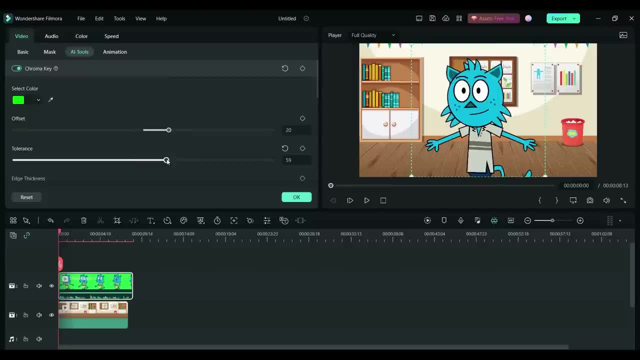 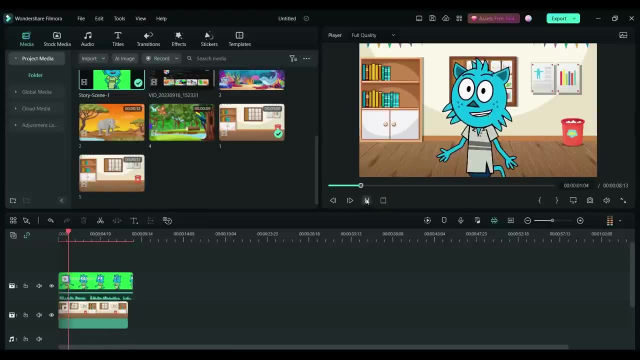 and if we drag it up a little bit, you'll notice that our character's shirt reappears, which is great, and now we can play around with exactly where we need this character. now you'll notice that i didn't adjust the length accordingly. filmora has the snapshot function, where you can actually just 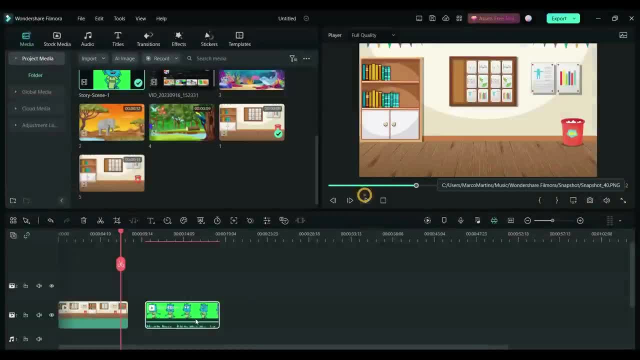 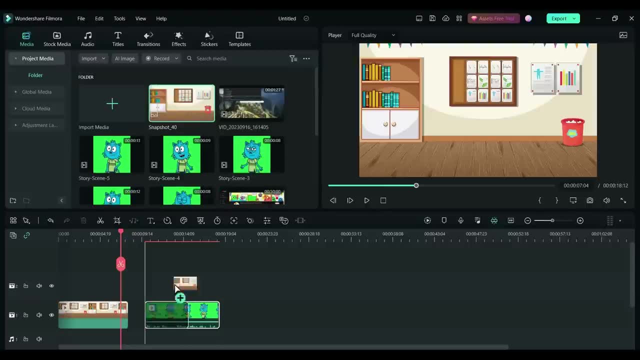 take a picture of your scene and luckily there's nothing moving in this picture, so all i need to do is take that snapshot- and i'm going to put it next to our timeline there- and just cut that piece out, and then you'll see it fits in beautifully. 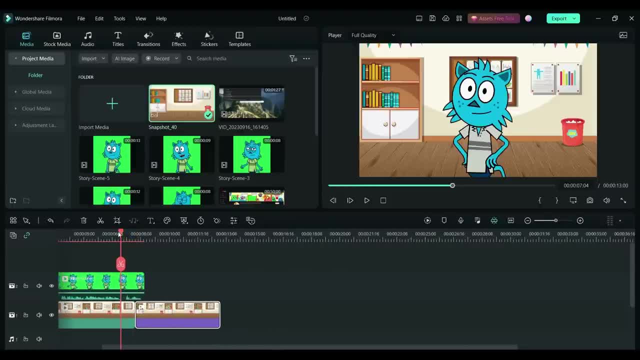 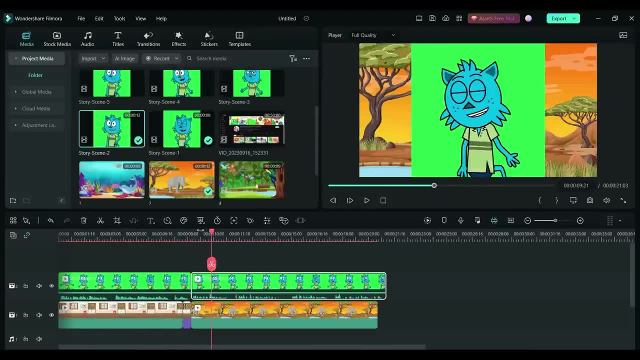 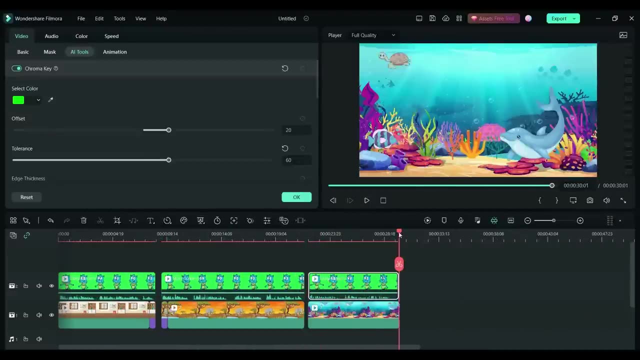 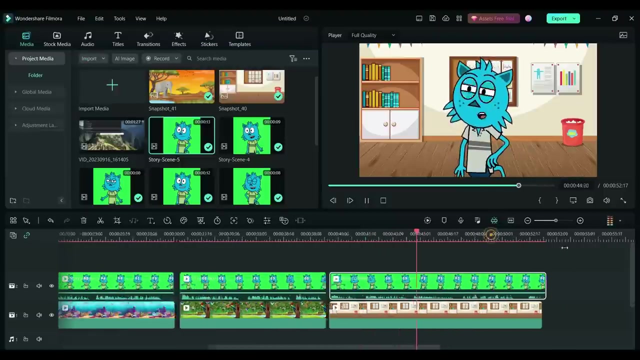 then we go to the next scene and we're going to do exactly the same thing: adjust the tolerance, make our character a bit smaller. wow, that is looking fantastic. i'm also going to put a bit of a gap between each of the scenes because i wanted to slow down a little bit. okay, so we do. 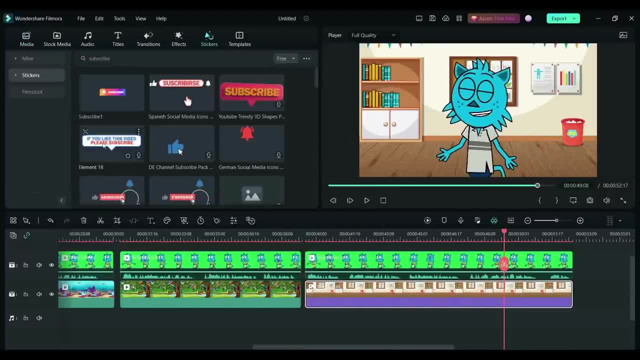 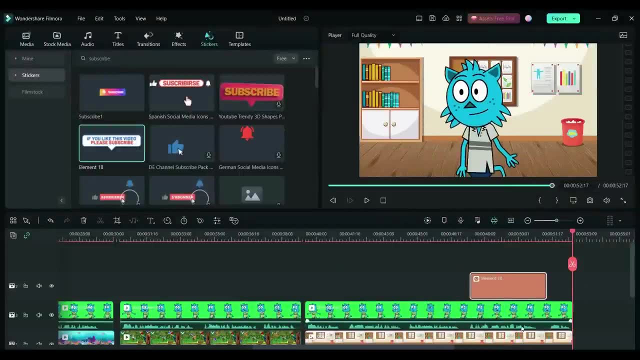 our final scene and then we're going to go to the next scene and we're going to do exactly the same thing. i'm going to make some minor adjustments. now, the cool thing about filmora here: if you go to stickers, you can add the different effects that you're going to. you're going to see, so you can. 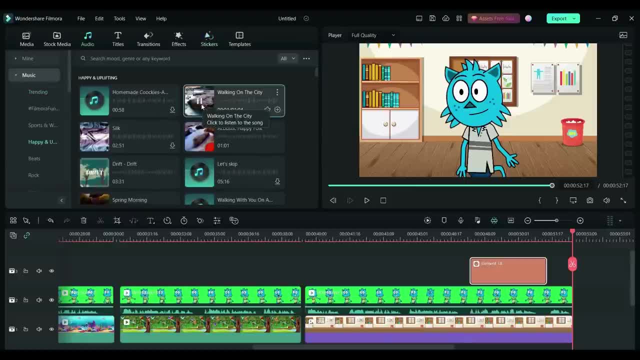 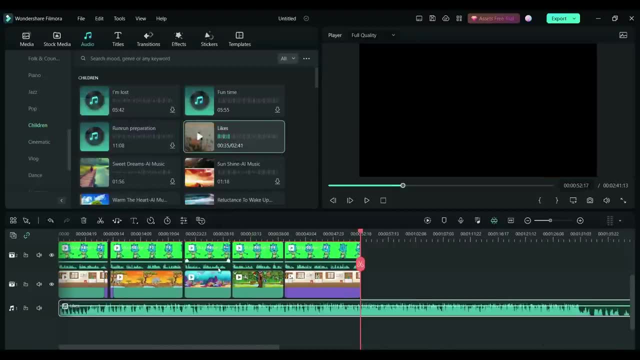 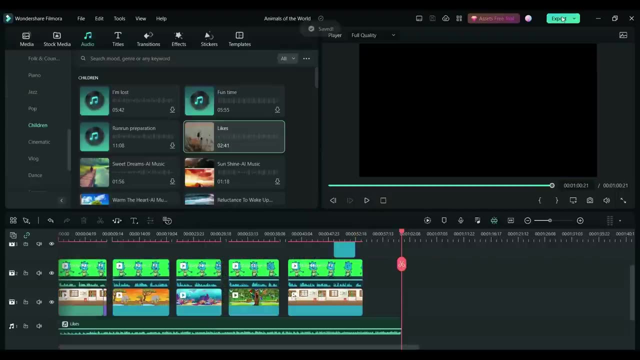 get people to like and subscribe once they've seen your video, and then we can add some music to it. so filmora has a great choice of children's music that we can use. these are for commercial use as well. once we're happy with everything, we can go ahead then and export it. now we can upload it. 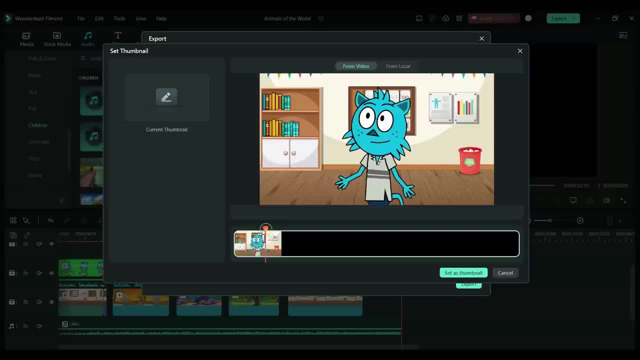 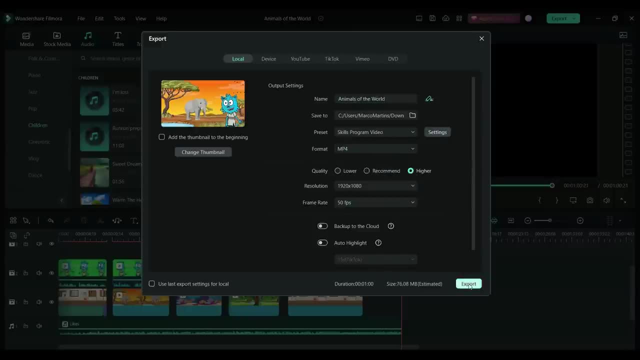 directly to filmora and then we can go ahead and export it. now we can upload it directly to filmora, to youtube, by putting in those details and adding a thumbnail, or we can save it to our computers as well, so we can add a general description. we're going to save it and let's have a listen to what. 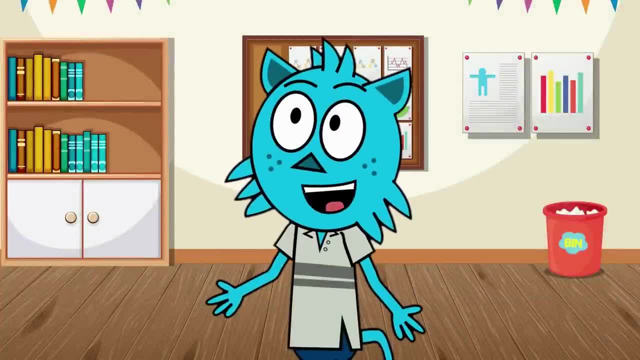 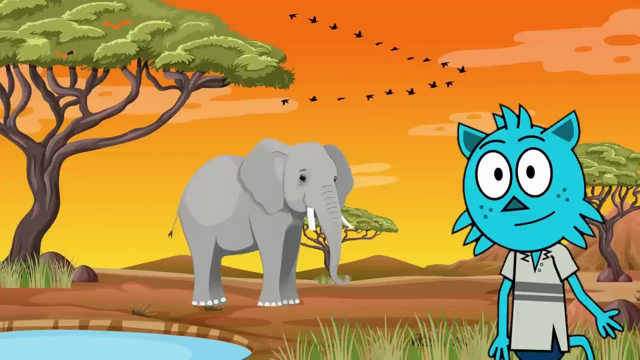 it's created. hello, young explorers. are you ready to go on a learning adventure? today, we will introduce you to three amazing animals from around the world. let's get started. our first stop is the african savannah to meet the elephant. did you know? elephants are the largest land animals. 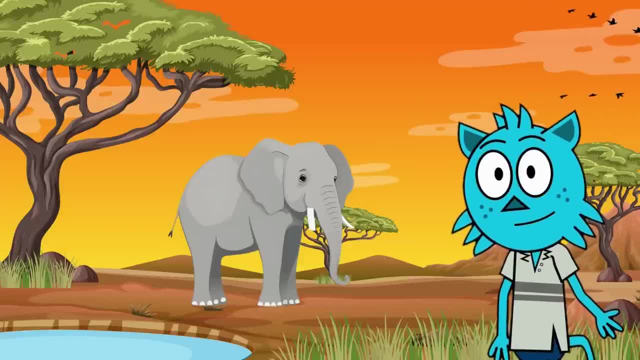 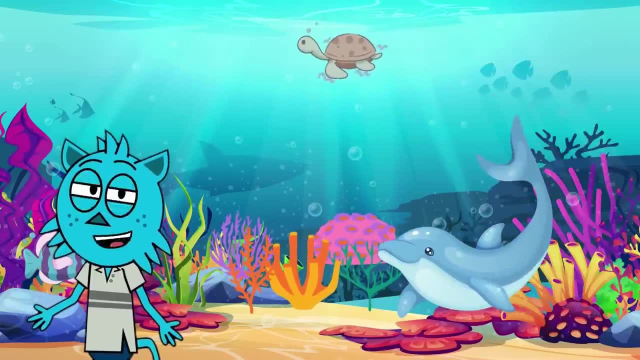 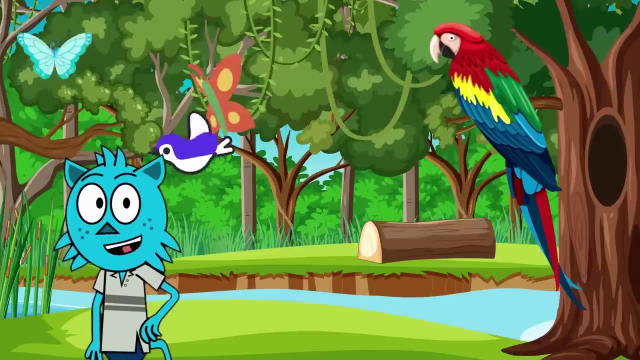 they love to eat plants and have big ears to keep them cool. next we're diving into the ocean to meet the dolphin. dolphins are very smart and social animals. they communicate with clicks and whistles. our last stop is the amazon rainforest to meet the colorful macaw. macaws are known. 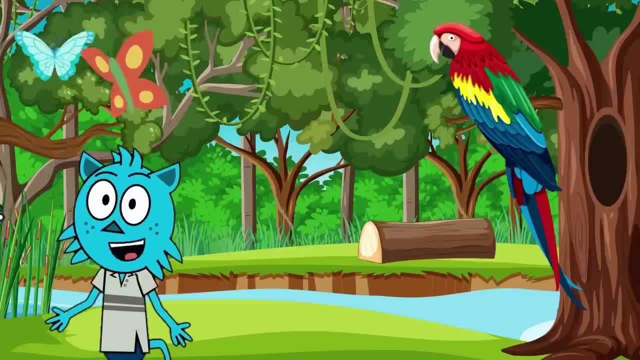 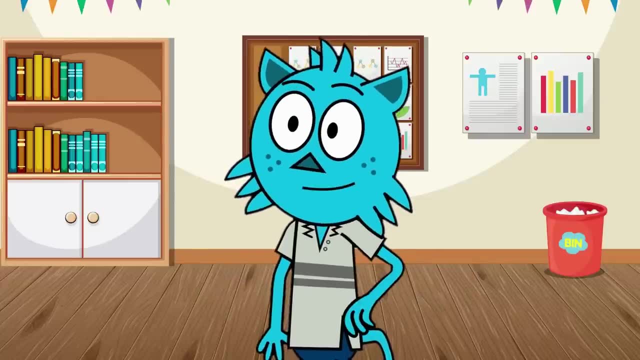 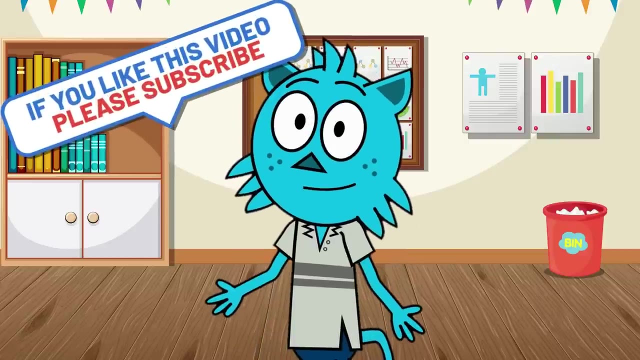 for their bright feathers and strong beaks. they love to eat fruits and nuts. and there you have it, explorers: three amazing animals from different parts of the world. thanks for joining us on this educational adventure. don't forget to like, share and subscribe for more fun learning. see you next time. oh wow, that is actually pretty, pretty cool. 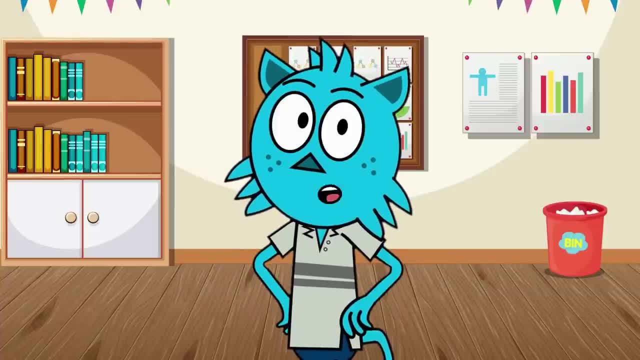 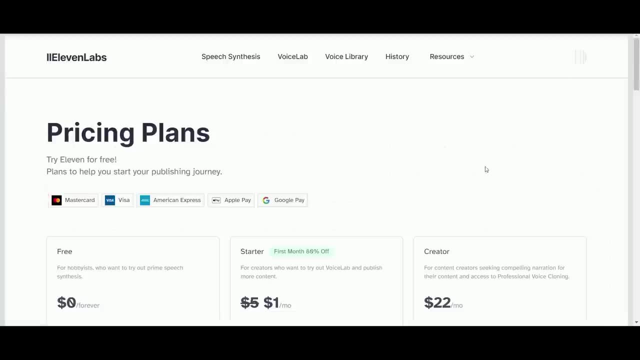 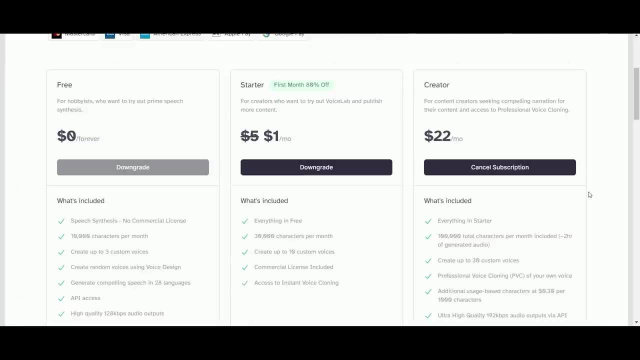 so, guys, there you have it. that is exactly how to create your own animation in under 20 minutes. just as a recap, i'm going to show you here. if we look at 11 labs pricing you're looking at currently a dollar per month for over 30 000 characters, but 10 000 characters per month for free. 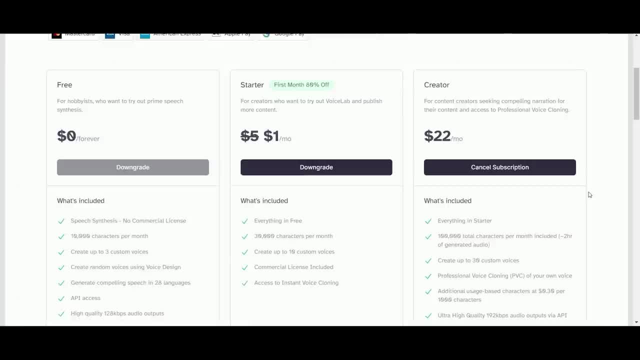 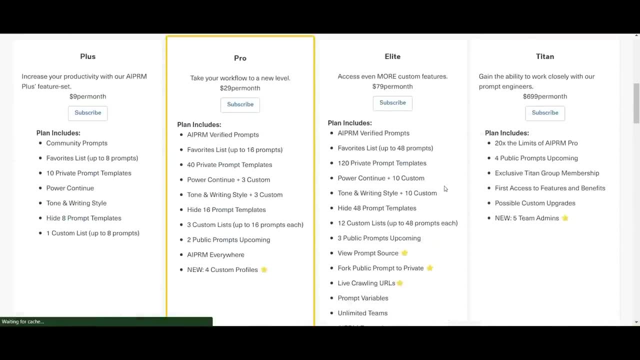 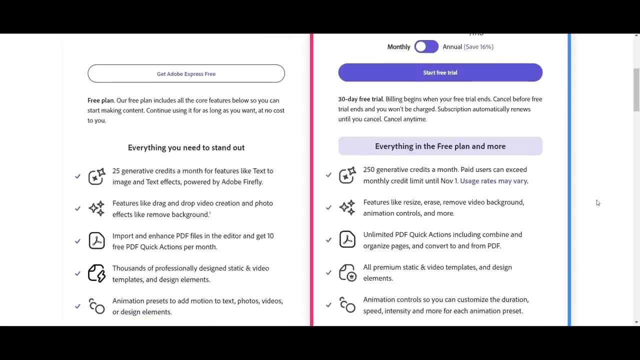 forever, which is more than enough for what we need for our animations. then aiprm has a prompt library for chat, gpt. it's kind of pricey but you can get away with the free version with plenty of functionality. and then adobe express you're looking at: wow, this is. this is a great tool and 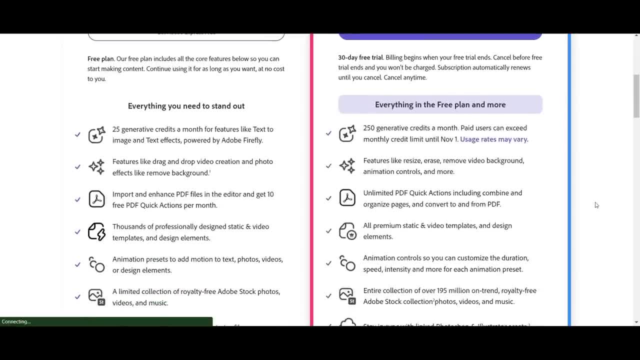 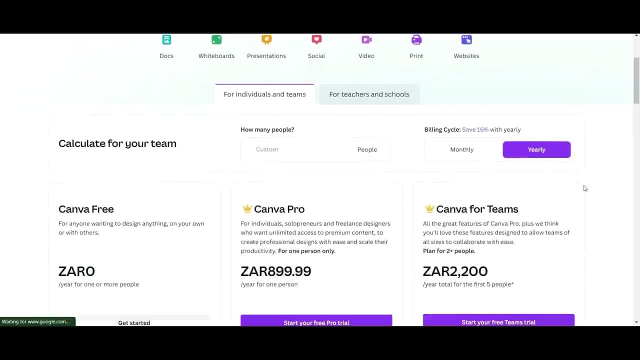 at ten dollars a month. you have access to those animations and a whole lot of other things that adobe is going to give you. so, wow, it's very cool. then we have canva. you're looking at about under ten dollars a month for the amazing things that canva can do. 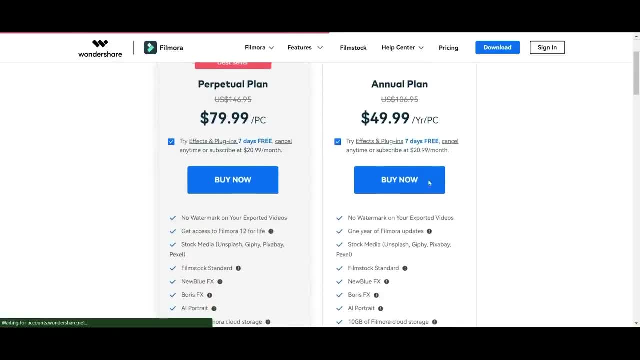 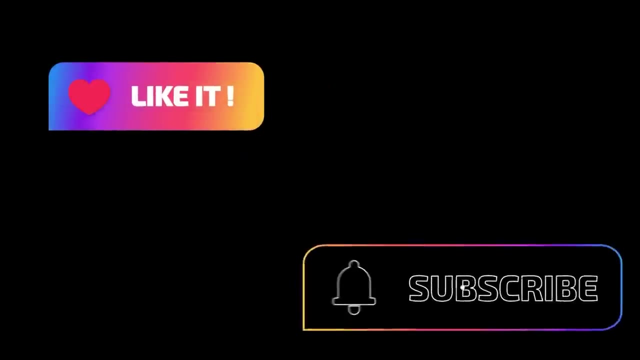 and filmora. you're looking at about eighty dollars for a perpetual license, so a once-off payment that will allow you to use filmora for the rest of your life on your computer. it is a steal. we hope that you guys have enjoyed this video. if you have, remember to like and subscribe for more content. just like this you.